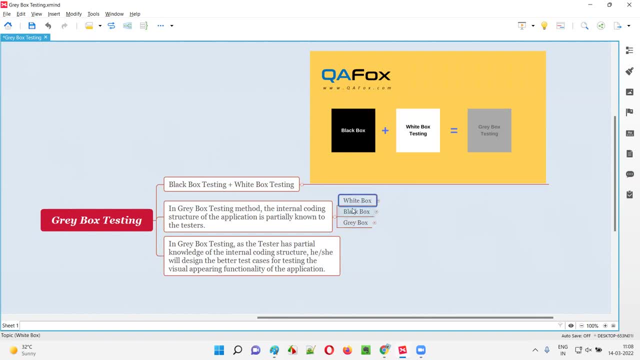 black box testing. Then you can understand what exactly is gray box testing. So let me first explain what is white box testing. In case of white box testing, a person who is performing this white box testing knows the internal code implementation in a full manner. The complete. 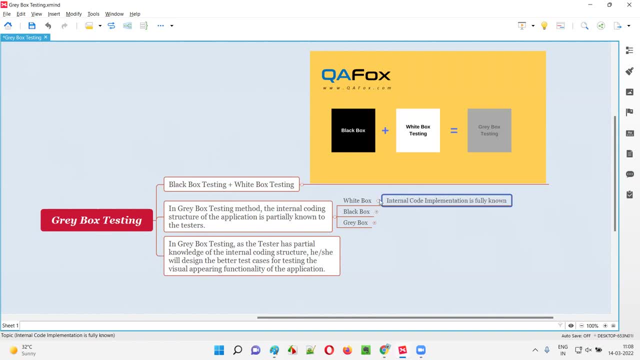 code that is used for developing the software will be known to the person who is performing the white box testing. that is white box testing, okay. What about black box testing? in black box testing, the person who is performing the black box testing doesn't know anything about the code that is used for. 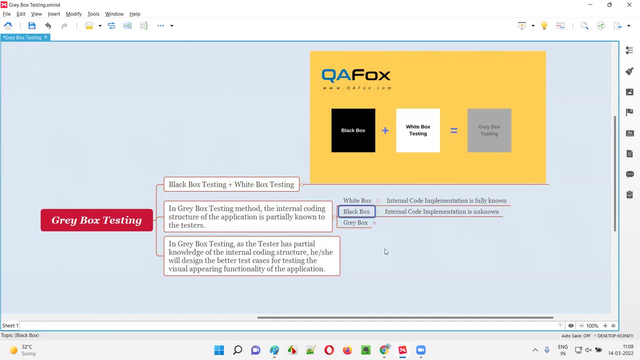 developing the software. instead, this particular person who is performing the black box testing will depend on the visual appearing functionalities of the software to perform testing. It doesn't know anything about the internal implementation of the code for developing the software. that is, black box Here, fully known. in case of white box, the internal implementation code is: 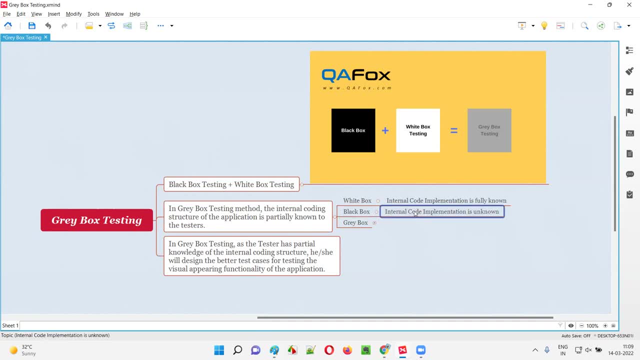 is fully known in case of white box testing. there is completely unknown in case of black box testing. okay, internal implementation code is completely unknown in case of black box. but in gray box it is partially known, here fully known. here is completely unknown, here partially known. guys, you know it partially. okay, the code that has been used for developing the software is partially. 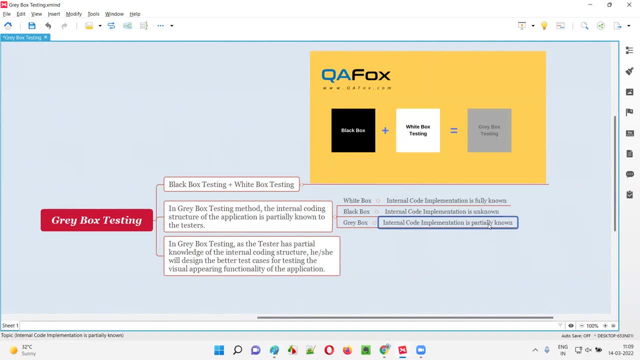 known. it's not completely known or entirely known, but it's partially known. okay, the pun who is performing the gray box testing will have some knowledge. okay, has some high level knowledge of what code has been written for developing the software. but he doesn't. he or she doesn't have the 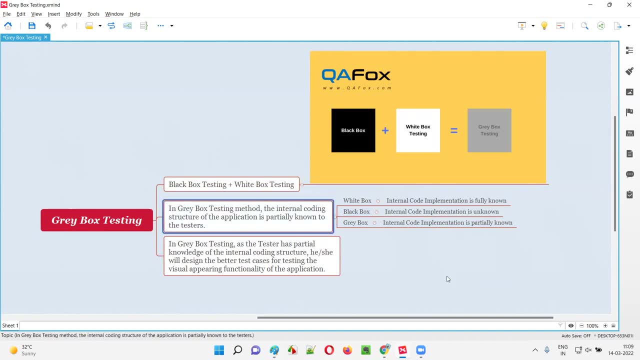 entire knowledge, but a partial knowledge is there. so what is the advantage, guys? okay, just to conclude, guys, in gray box testing method, the internal code structure of the application is partially known to the tester who is performing the gray box testing. okay, it's here. it is partially known. so what is? 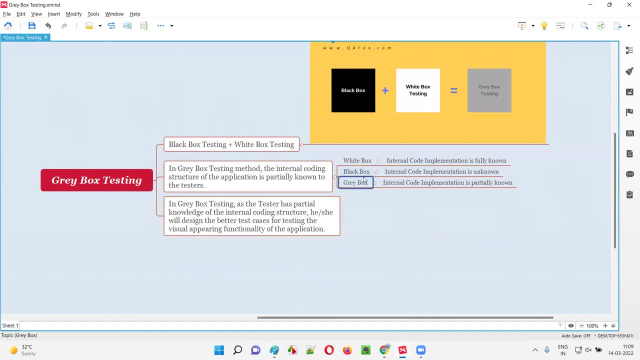 advantage? okay, what is advantage advantage of the gray box testing over the black box testing? in case of black box testing, right, we only test the software by depending on the visual operating functionalities of the software, right? so the one who is performing black box testing will will create some test cases in 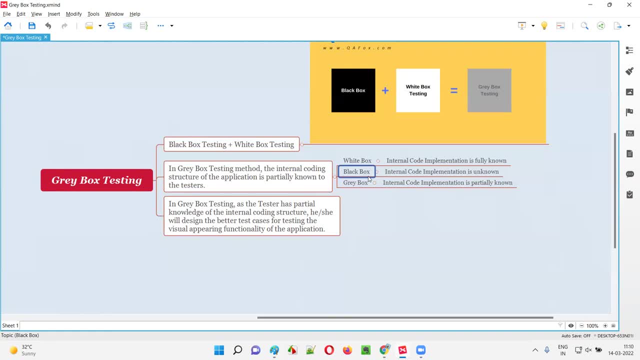 advance. right, you will not directly perform the testing, right? he, he or she has to create some test cases to perform the black box testing. but in case of gray box testing, the person who is performing the gray box testing has partial knowledge of the internal code implementation of the software.